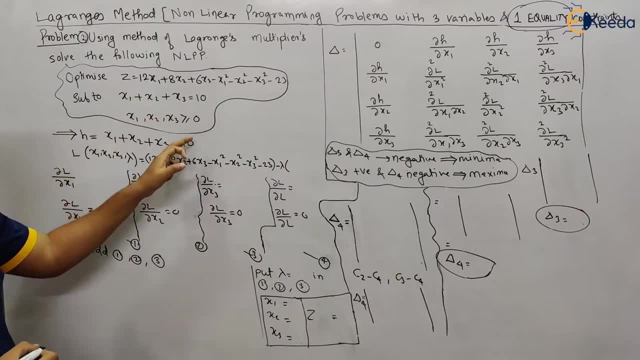 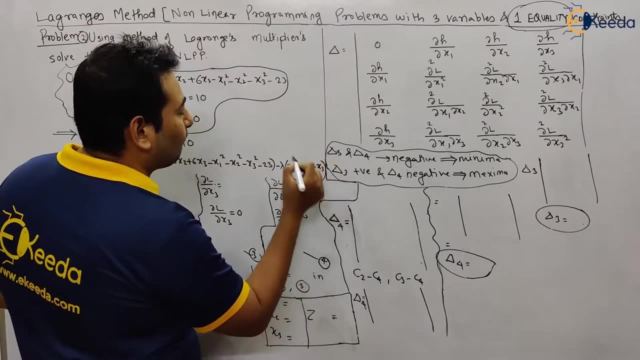 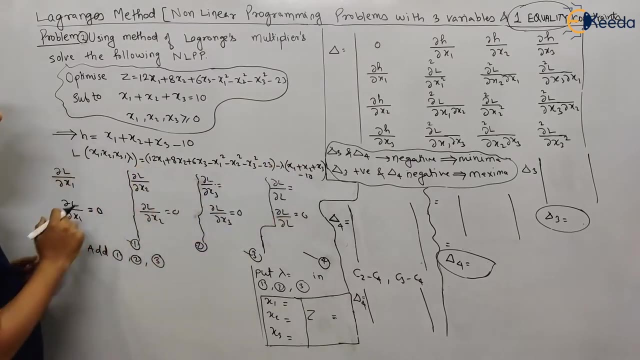 minus lambda time constraint. And what is the constraint? This is the constraint, that is x1 plus x2 plus x3 minus 10.. So this is the constraint. Let us quickly find out the things. Dual upon dual x1.. Let us differentiate with respect to x1.. So this: 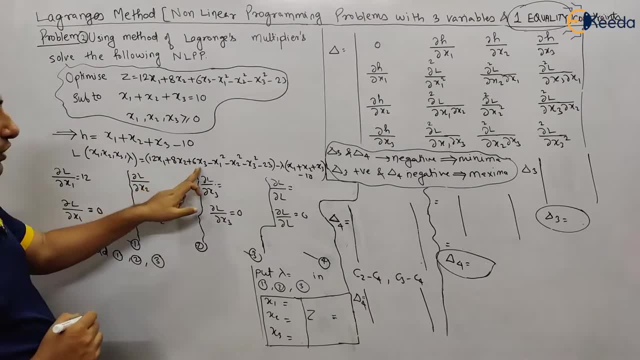 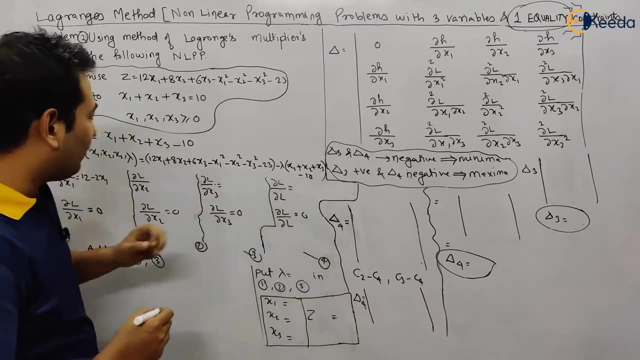 will be 12.. 0, 0. this is minus 2 x1.. This is 0: 0 and from this we'll get minus lambda. Let us differentiate with respect to x2 partially. So this is 0: 0 and from this we'll get minus lambda. 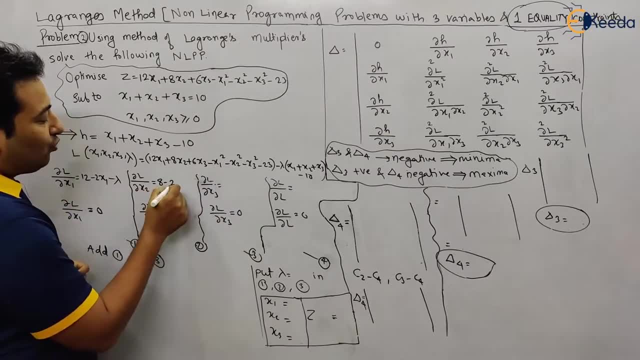 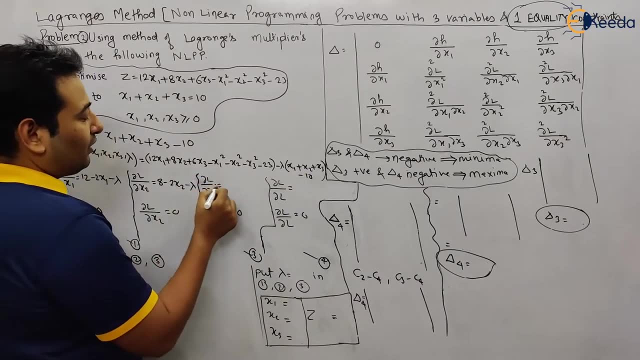 This is 0, this is 0. here it is 8. this is minus 2 x 2, and then from this we'll get minus lambda. Next with respect to x3.. With respect to x3, you will get 6, then minus 2 x 3, and then 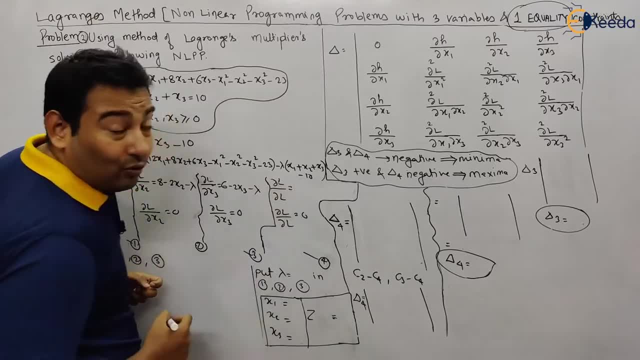 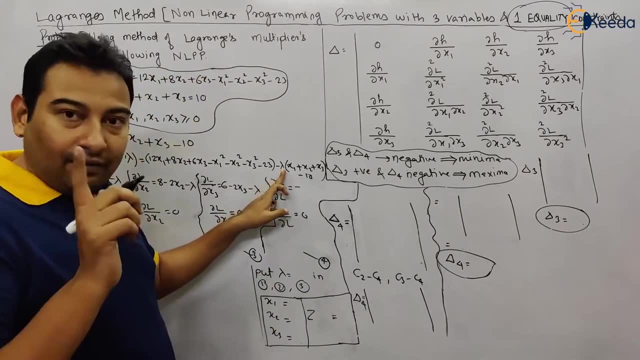 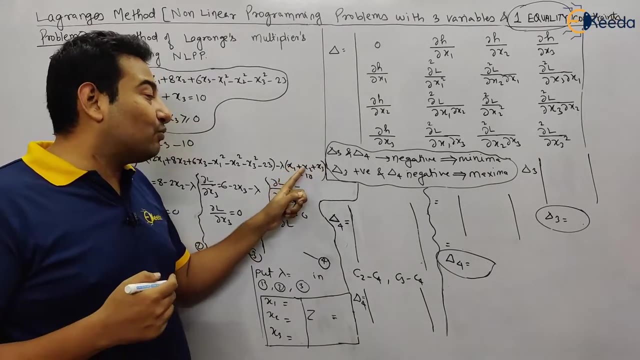 minus lambda. and finally, with respect to lambda, if you gonna differentiate, so this will be minus. see this: minus lambda derivative is 1 and this term will remain as it is. that is x1 plus x2 plus x3 minus 10. so minus will go inside. that will become minus x1 minus x2 minus x3 plus 10. 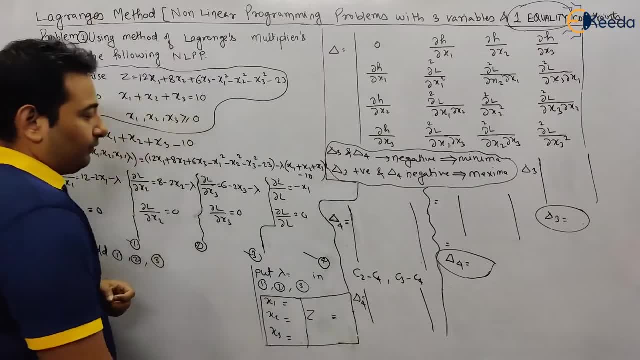 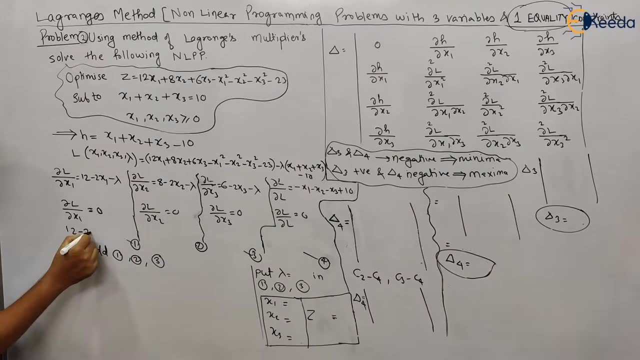 what next? let us equate it to 0, so this will be: 12 minus 2 x1 minus lambda, equal to 0. this is equation number 1. 8 minus 2 x2 minus lambda, equal to 0. this is equation number 2. and finally, 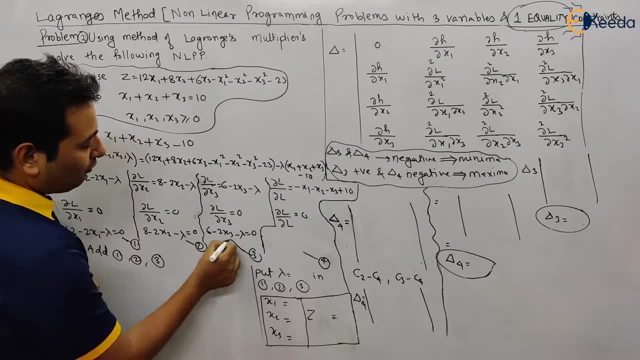 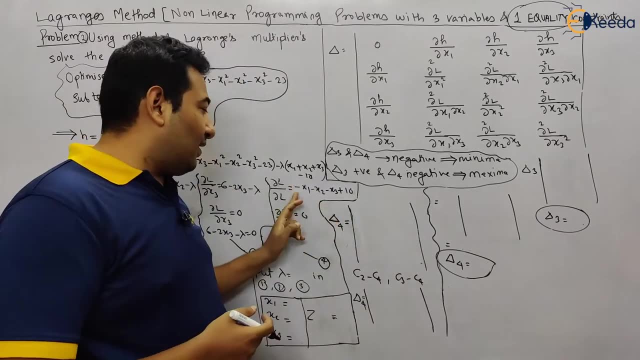 6 minus 2, x3 minus lambda, equal to 0. this is equation number 3 and here, if you equate it to 0, 10 will go to that side and will become minus 10. see, all are minus if you multiply by minus. 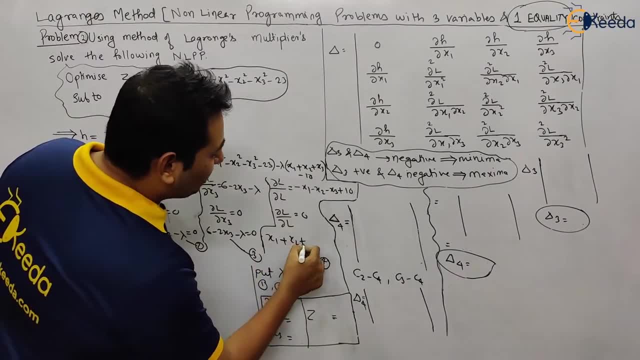 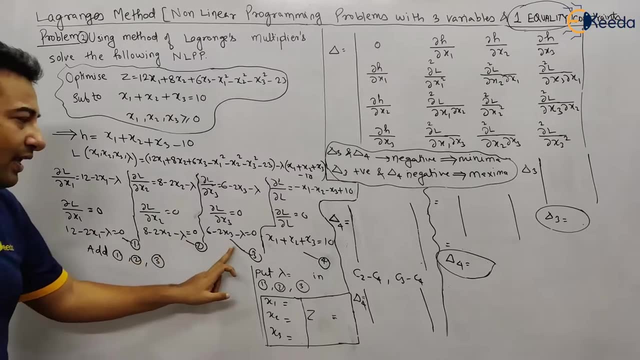 everything will become plus and it's simply x1 plus x2 plus x3 equal to 10. this equation number 4, as discussed, always fixed. you add these three equation and use equation number 4. this is fixed. add 1, 2 and 3. if you add 1, 2 and 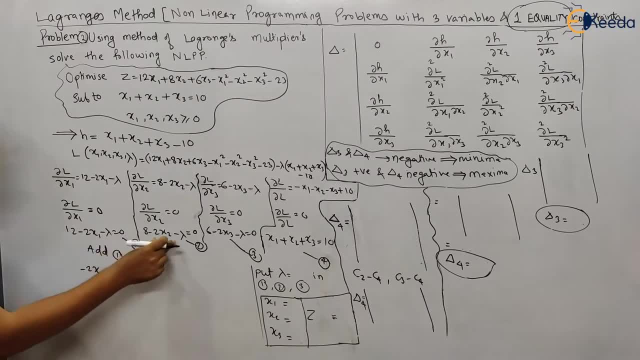 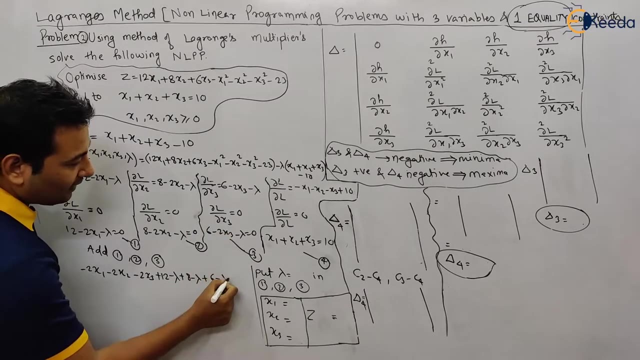 3, you will get see minus 2 x1 from this, minus 2 x2, minus 2 x3 and 12 minus lambda, 8 minus lambda, 6 minus lambda equal to 0. if we take minus 2 common from this inside, we'll get: 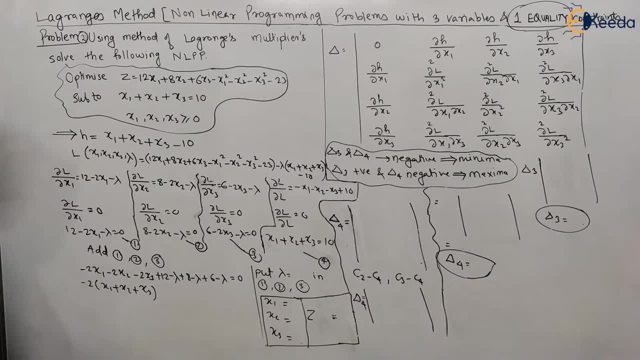 x1 plus x2, exactly similar problem. plus x3, this is 12, 8 and 6, that is 26 minus 3 lambda equal to 0. so let us put this from equation number 4: the equation number 4- so this is a value- is 10. 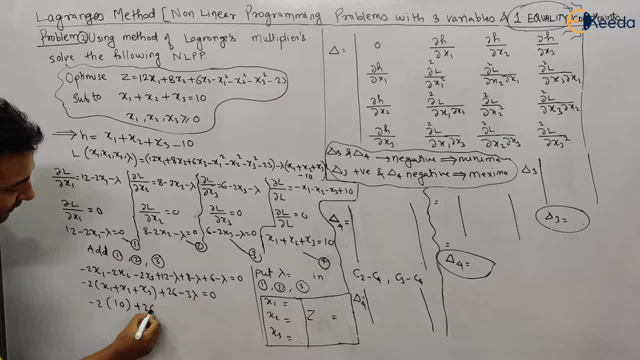 plus 26 minus 3: lambda equal to 0. so this is minus 20 plus 26. is what? 6 minus 3? lambda equal to 0. in short, lambda equal to 2. we got lambda equal to 2. what next we need to put in equation? 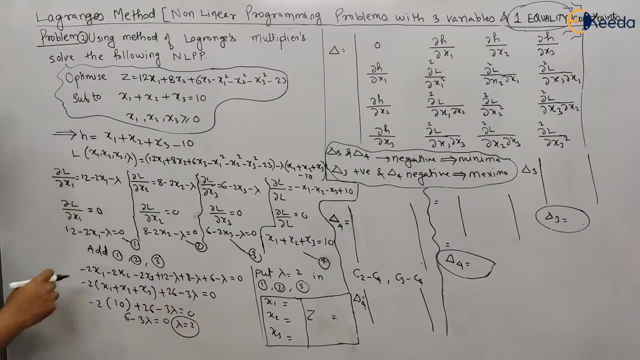 number 1, 2 and 3: see exactly similar procedure. if we put lambda is equal to 2 here, so this will be 12 minus 2, that is 10 minus 2. x1 plus 10, that means x1 is equal to 5. next, if i'll put lambda is equal, 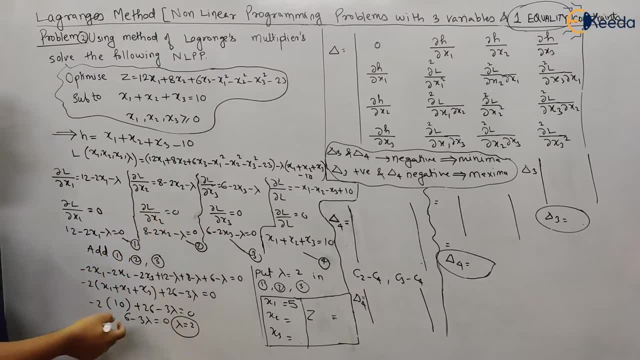 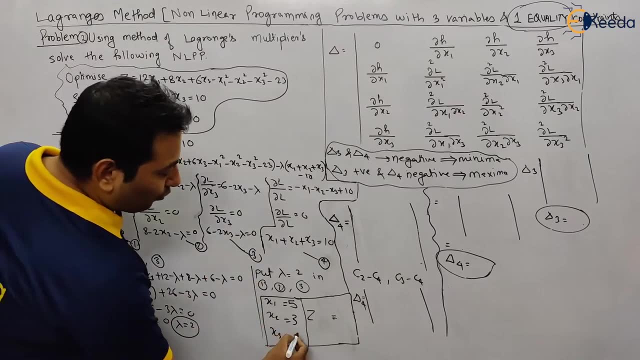 to 2, so 8 minus 2 will be 6. we'll go to that. 6 x2 will be 3 and if we put lambda is equal to 2 here. so 6 minus 2 will be 4 and 2. so these are the values of x1, x2, x3. you can check once you can. 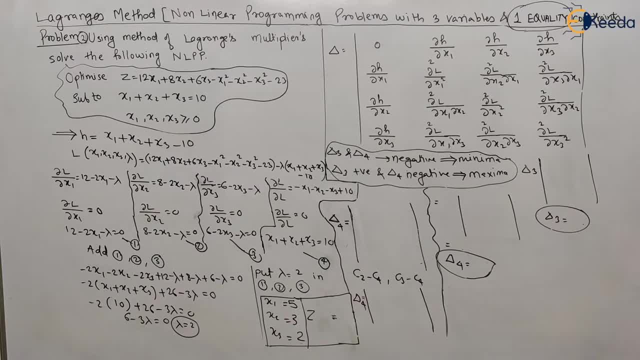 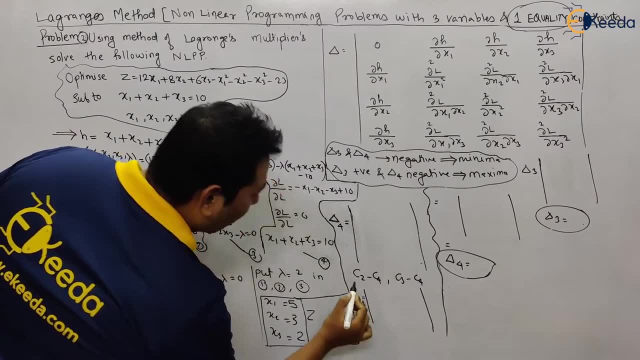 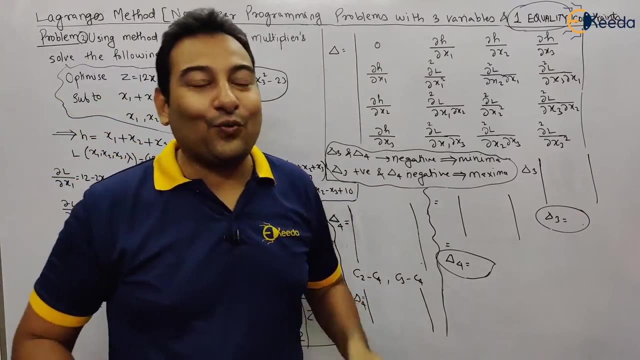 verify the values and if you put all these values in equation number 1- x1, x2, x3, in equation number 1, z value we're going to get is 35. the only thing that needs to be checked is whether it's a maximum value or minimum value for that purpose. we know what to do. use of this hessian matrix. 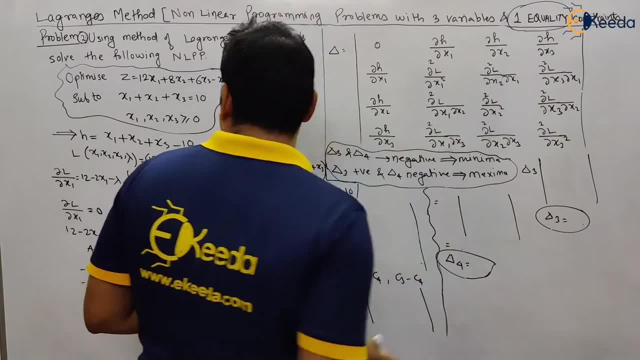 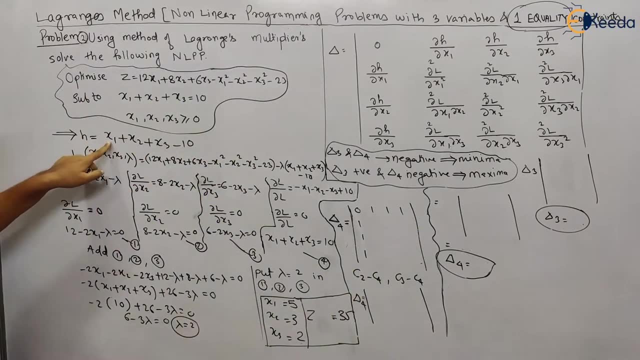 so here it is 0. next, h: x1, x2, n, x3. so if you differentiate with respect to x1- hope this is clear- with respect to x1, x2, x3, if you differentiate this, you will get 1, 1, 1. what next? we already have doul upon 2 x. 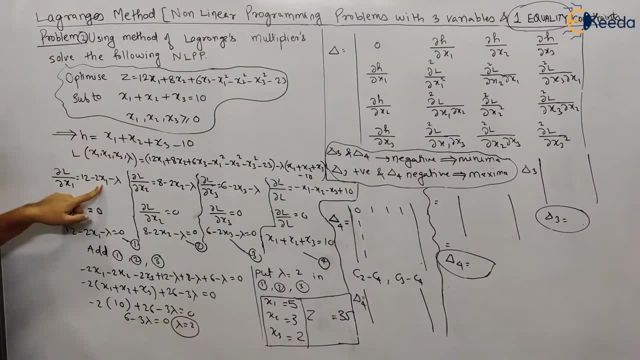 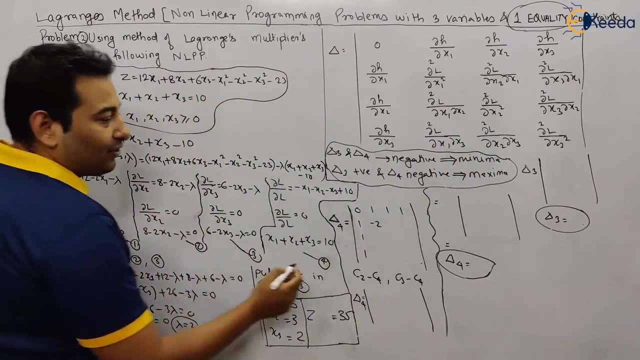 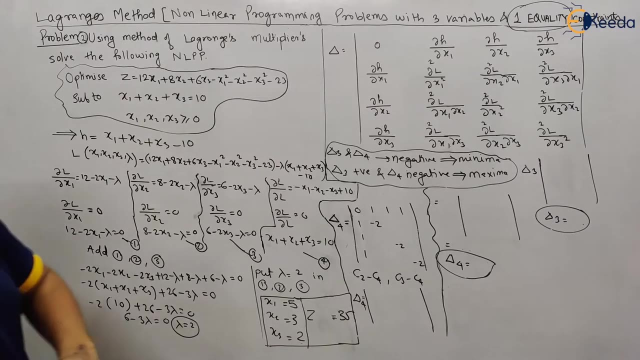 1. we need to take differentiation with respect to x 1 again, so that is minus 2. if we differentiate with respect to x 2 for this term, again minus 2 and minus 2. remaining all the terms will be 0. how see here x 2 and x 1? we already have x 1. 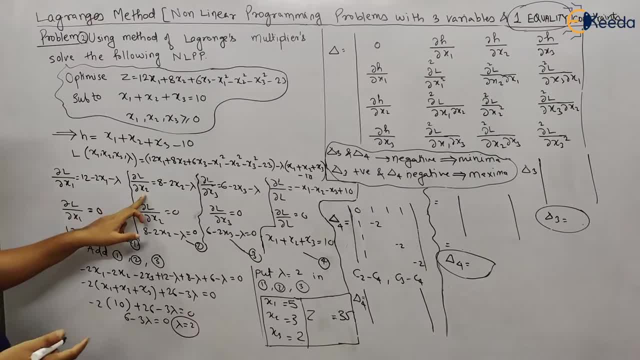 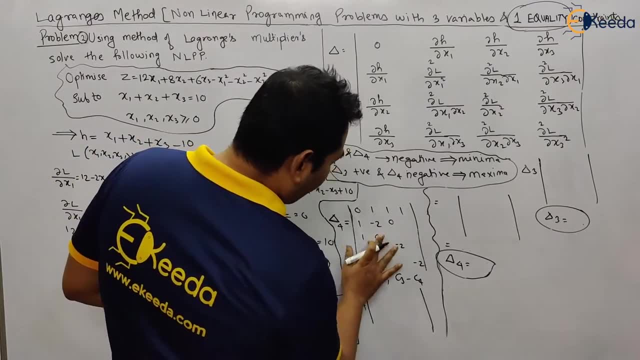 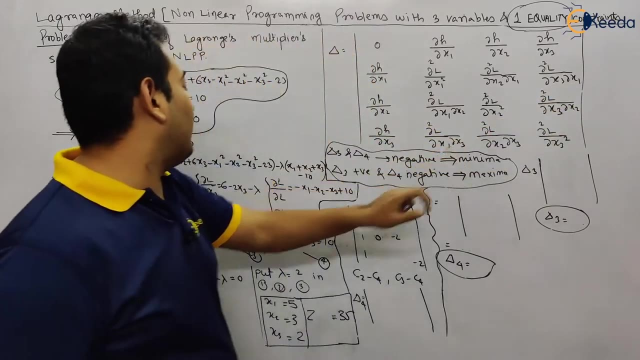 and if you differentiate with respect to x 2: 0. if you differentiate, so this will be 0, here it will be 0. what next see here? x 3, x 1, x 3 x 1, so x 1. if you differentiate with x 3, again it is 0. 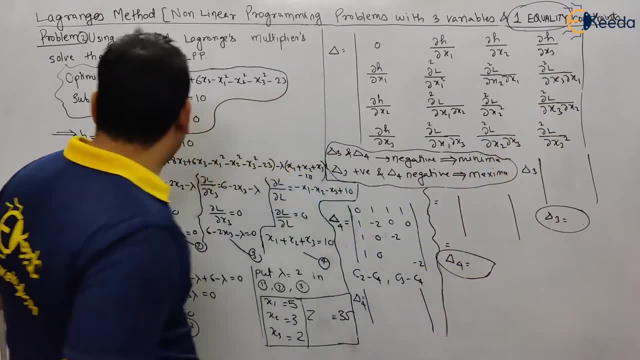 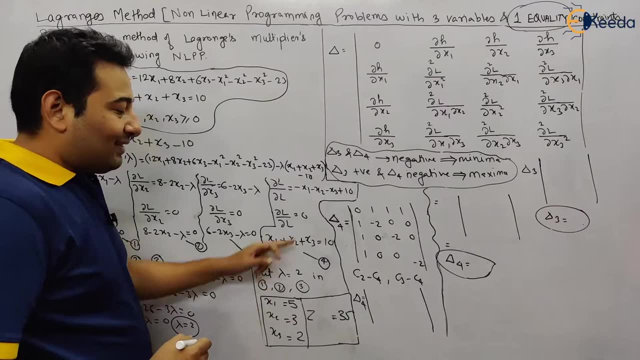 so here it will be 0. and finally, x 3 x 2. so if you differentiate x 3 with x 2, again it will be 0. so this is the matrix. this is a delta 4. delta 3 will be a 3 cross 3 matrix. 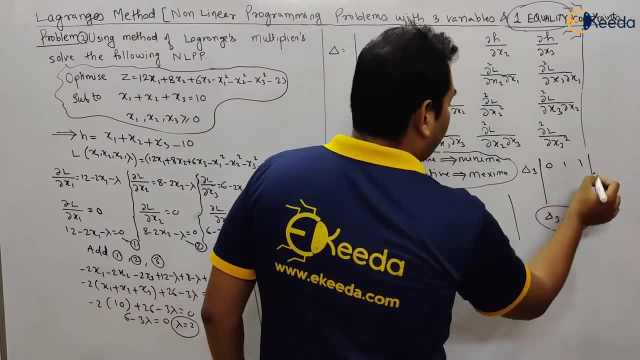 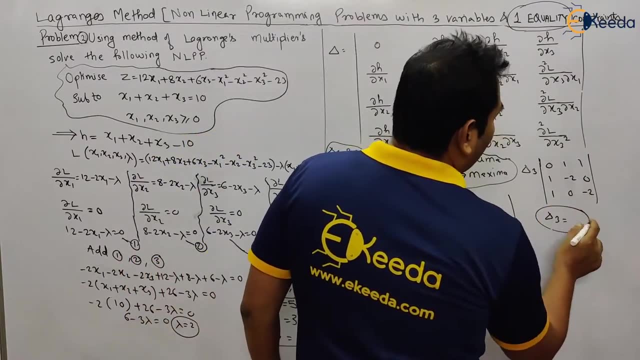 so you need to take first 3 rows and columns. so you need to take first 3 rows and columns. that is 0, 1, 1, 1 minus 2 and 0 and finally 1, 0 minus 2. if you solve, you will get delta 3 value is a 4. 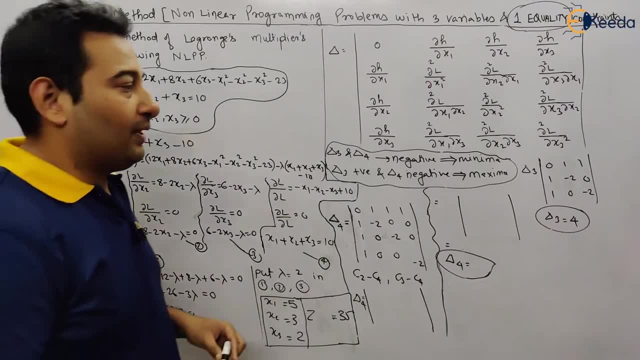 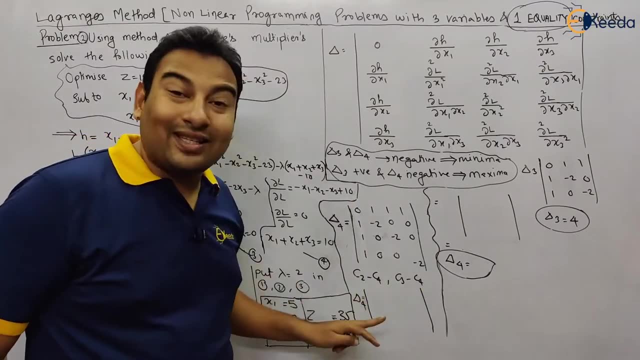 you can try doing it. you will get the value as 4. let us find it out. delta 4, delta 4: is this again the same procedure: c 2 minus c 4, c 3 minus c 4, c 2 and c 3 will change. c 1 will remain same. 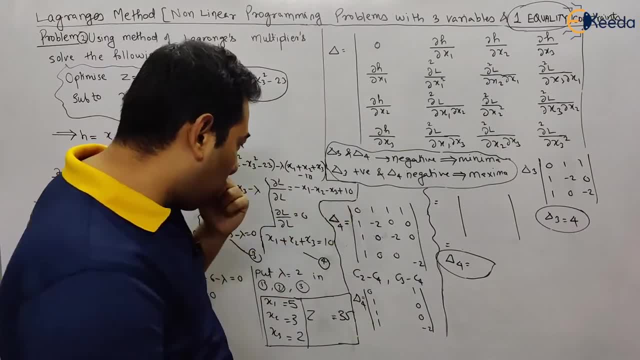 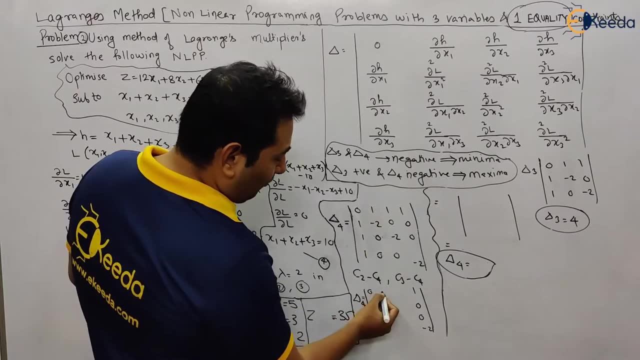 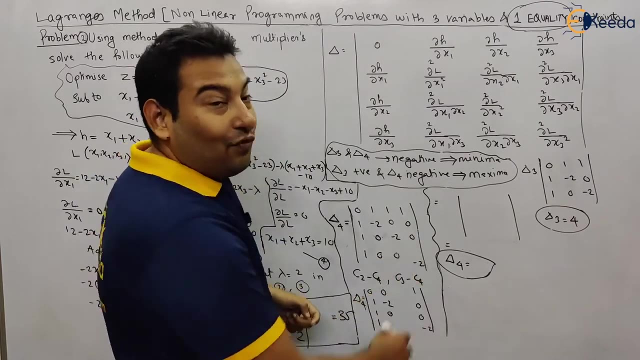 c 2 minus c 4 and c 3 minus c 4. c 2 and c 3 will change: c 2 minus c 4, 1 minus 1 0 minus 2 minus 0 minus 2. 0 minus 0, 0, 0 minus of minus 2. that will become plus 2. 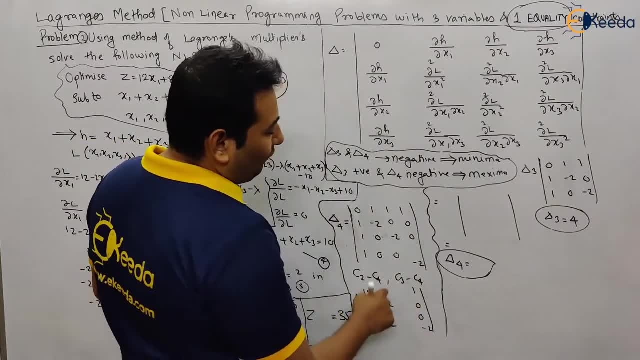 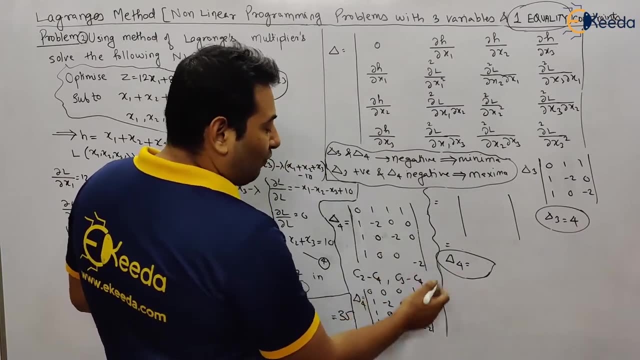 next: c 3 minus c, 4, 1 minus 1, 0, 0 minus 0. 0 minus 2 minus 0 minus 2. 0 minus of minus 2, that will become plus 2. minus of minus 2, that will become plus 2. again, the same story: minus 1 will be outside.